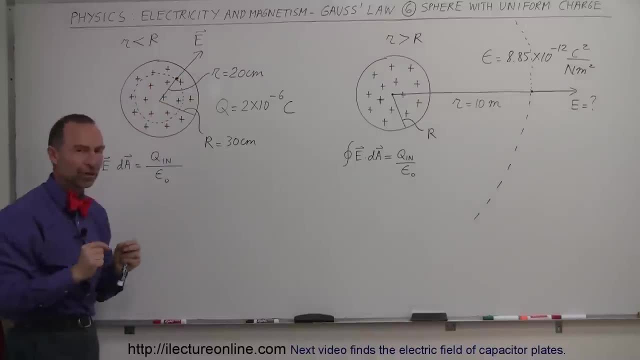 where the edge of the surface is right, at the point where we want to know the electric field strength, Realizing that the electric field will always be perpendicular away from that Gaussian surface pointing outward, and will be exactly the same strength everywhere along that surface. that's. 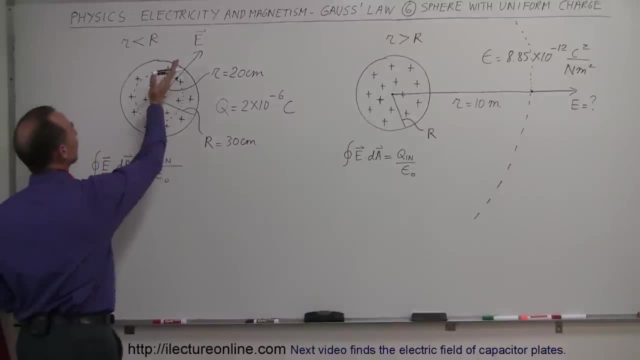 why we can use Gauss's law like this. So since the electric field will be perpendicular to the Gaussian surface, this part of the equation simply becomes: the strength of the electric field times the area, the total surface area of the Gaussian surface. so let's call that a and that. 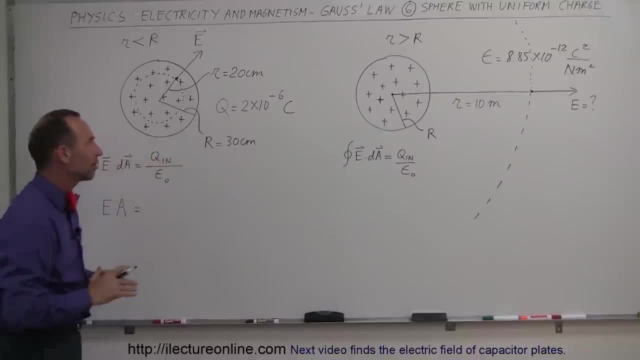 equals the charge inside divided by epsilon sub naught. So how much charge is now inside the Gaussian surface? Well, we're given the charge inside the whole sphere. so we have to find the ratio of how much is inside the Gaussian surface compared to inside the whole sphere, and that simply will be the ratio. 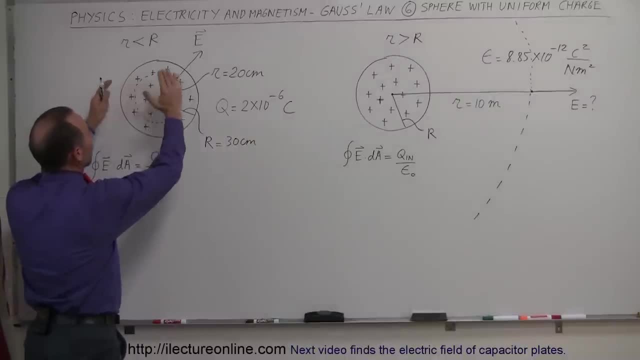 of the volume of the Gaussian surface divided by the volume of the whole sphere. So this becomes the total charge q 2 times 10 to the minus 6 coulombs times the ratio of the volume of the Gaussian surface divided by the volume of the sphere. and so now we can plug in what these things? 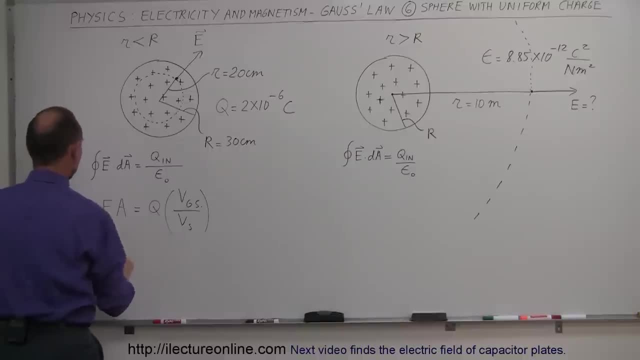 are equal to, So in this case that would be e times the area. the area of the Gaussian surface will be four pi r squared, r being the radius of the Gaussian surface. and of course, the surface of a sphere is simply four pi r squared. that equals the total charge q times the ratio of the volume. 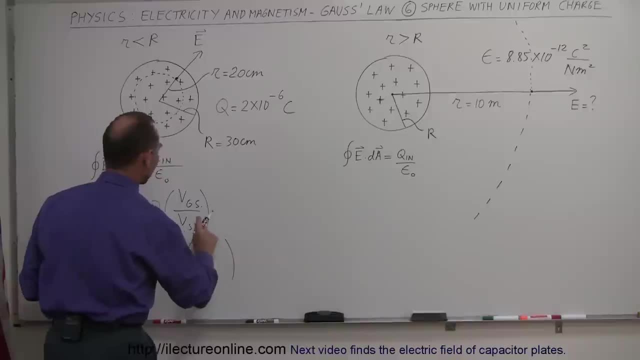 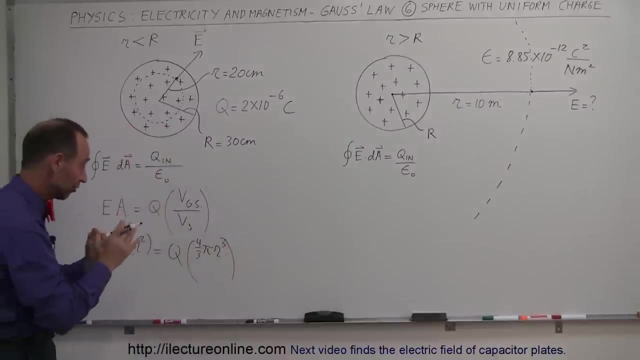 of the Gaussian surface, which is four thirds pi times the radius of the Gaussian surface cubed, which is r cubed. that's the volume of the Gaussian surface sphere divided by four thirds pi r cubed r, of course, being the radius of the whole sphere. notice that the four 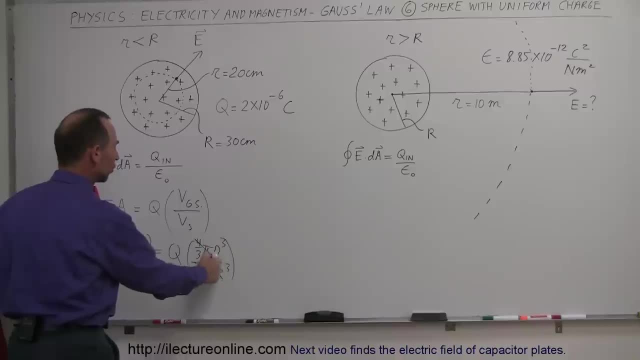 thirds, pi cancel out right here. and then we have simply the ratio of r cubed r, being the radius of the Gaussian surface cubed, divided by r cubed r big R being the radius of the whole sphere cube. and that ratio will give us the total charge inside, and of course we still have to divide it by. 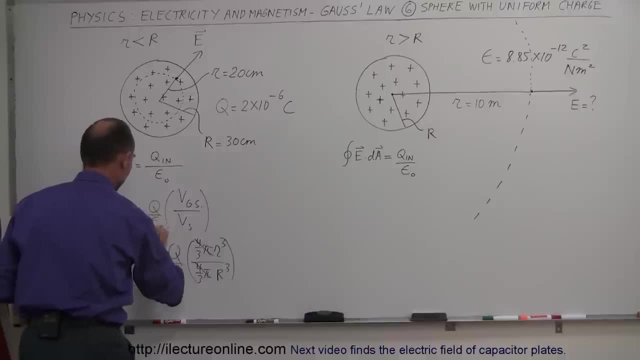 epsilon sub naught, and of course here I make sure that I put epsilon sub naught there as well, can't I put epsilon sub naught? all right, then all we have to do is go ahead and take this and solve this for e, and so we have the electric field. e is equal to. I don't have a lot of room there, so I'm going. 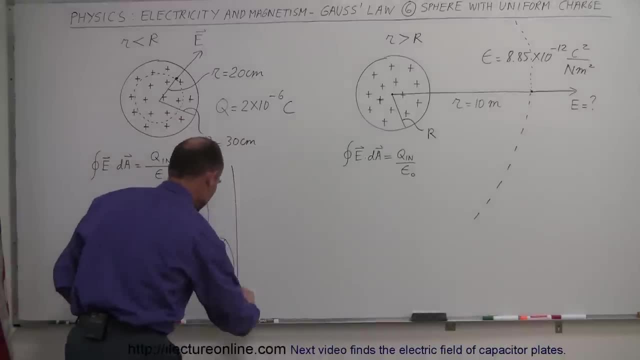 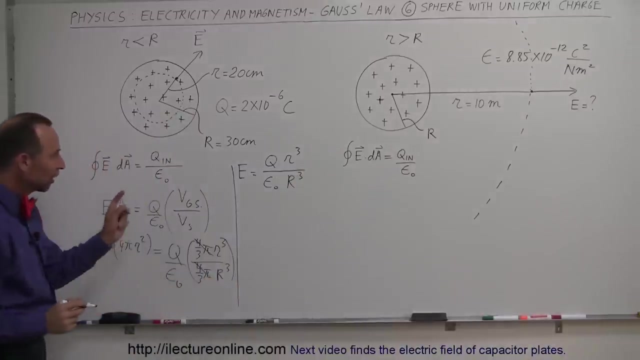 to migrate over in this direction. so let's put a line here, and so we're going to follow. continue here. so e is equal to the charge q divided by epsilon sub naught times, little r cubed divided by big R cubed. and then the four pi r squared is also going to go on the denominator. 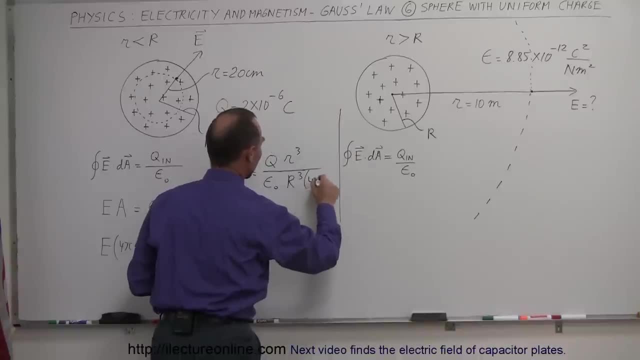 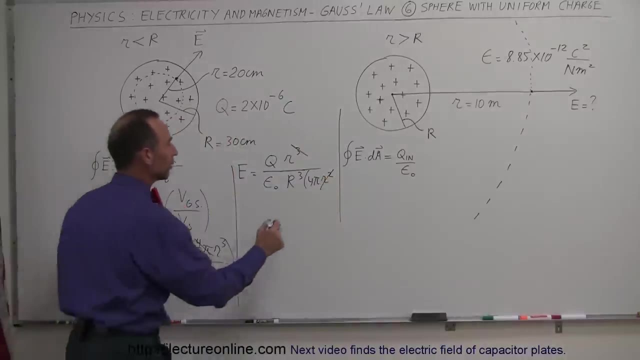 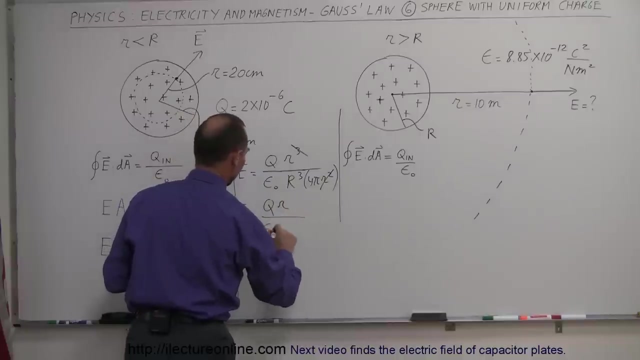 So here we go. this will be times four pi r squared, and of course this r squared will cancel out two of those, so only leave left with one r in the numerator, and so finally we can say that the electric field is equal to q times r divided by epsilon sub naught times four pi r cubed. 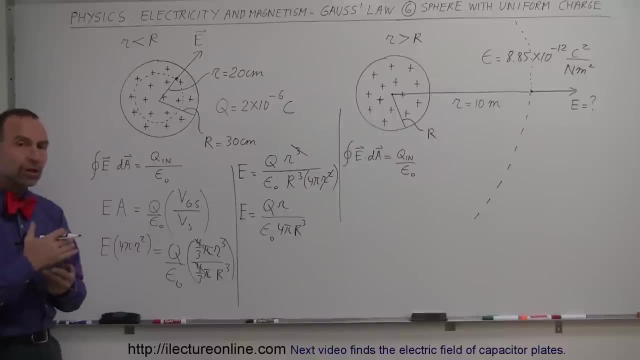 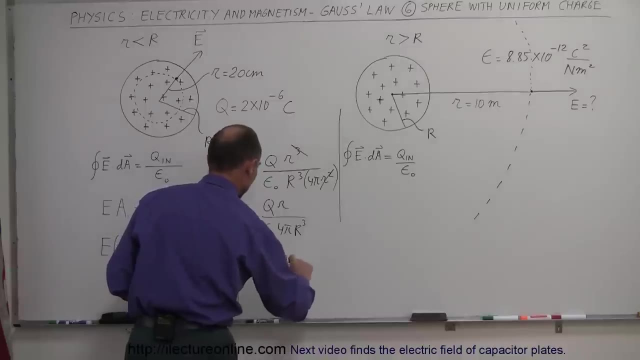 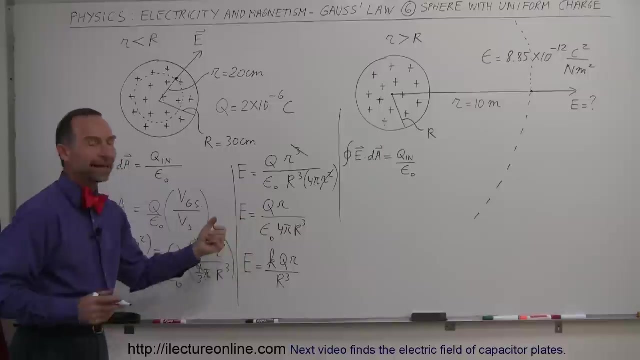 now, four pi epsilon sub naught is also equal to k, the constant we used in the coulomb's law. so it then has: e is equal to k times q, times r divided by r cubed. so either way, whichever way you prefer, remember that k is simply one over four pi epsilon sub naught, and k, of course, is at nine, point nine. 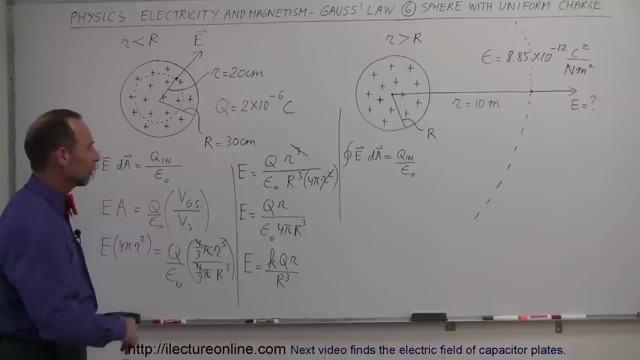 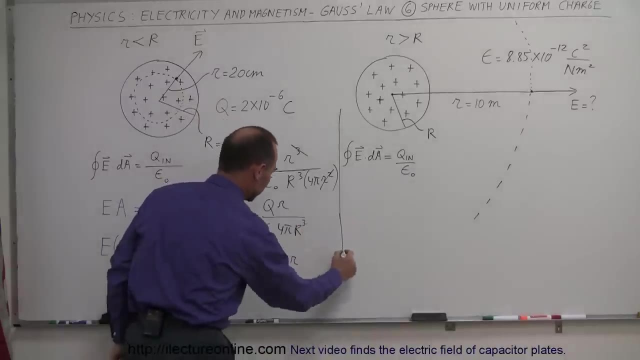 times ten to the ninth newton's meter squared per coulomb squared. all right, so now, if we want to put some numbers in there, we can go ahead and do that, but since I have not a lot, not a lot of room, I'll just leave it as is. so this is simply the result of the electric field. 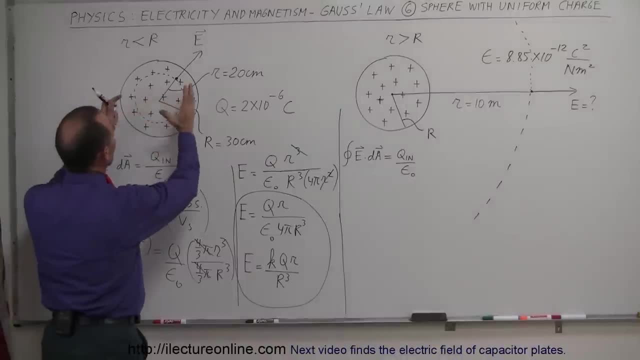 Now we're going to do the second part of the problem, where we try to find electric field strength inside a sphere that has uniform charge throughout the entire sphere. Okay, now we're going to the second part of the problem, where we try to find electric field. 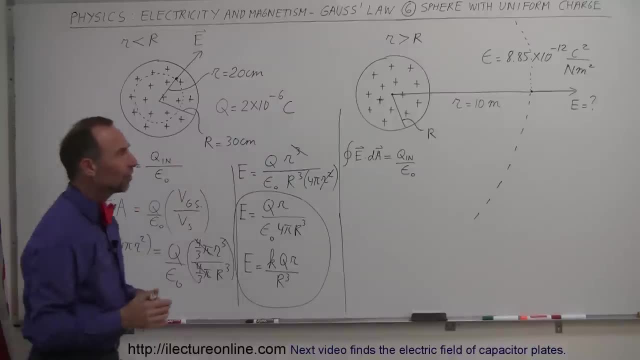 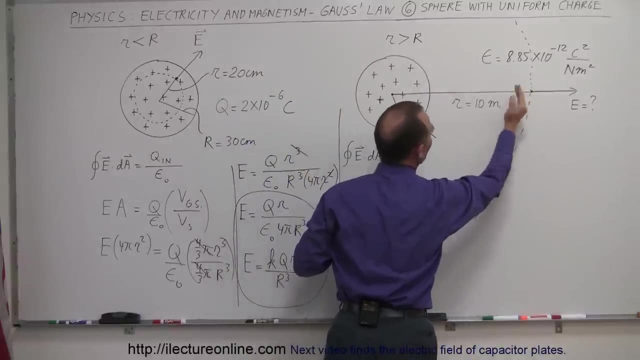 strength outside the sphere. now what happens is we're going to draw a really big gaussian surface, one that has a radius of 10 meters, in this case, and so that the electric field will be right on the surface again. since it's symmetrical, the electric field direction will always be perpendicular. 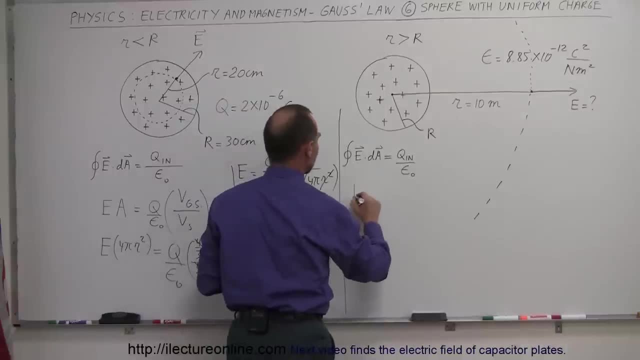 away from the surface. So using this equation right here, we can say that e the electric field strength anywhere along the gaussian surface times the total area of the surface, which will be 4 pi r squared, that's the surface area of a sphere. remember, in this case little r is bigger than big r. little r is all.